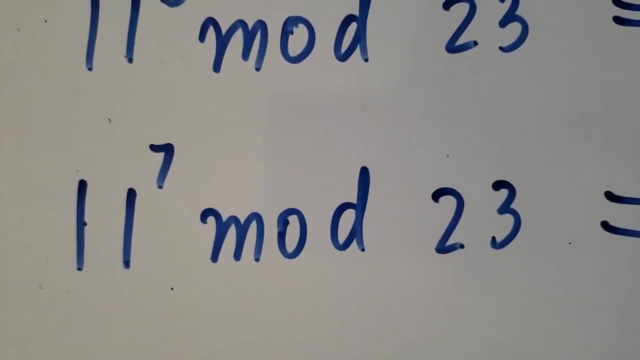 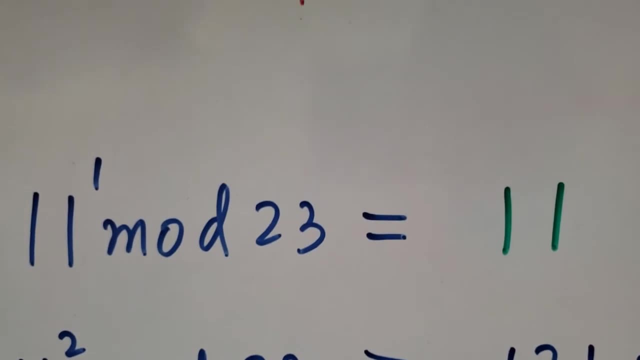 11 to the power 6 and 11 to the power 7.. We can go further if needed, but for now I'm going to go till 11 to the power 7.. So let's start with 11 to the power 1.. 11 to the power 1, mod 23 is 11.. 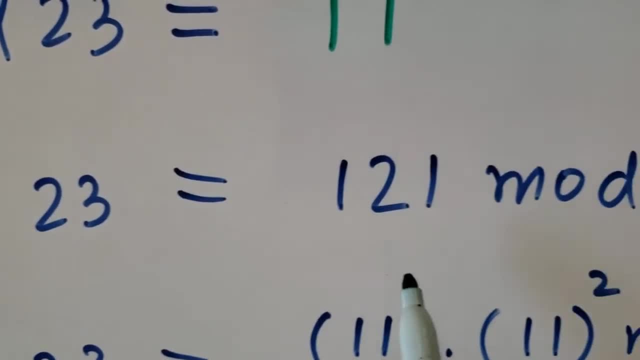 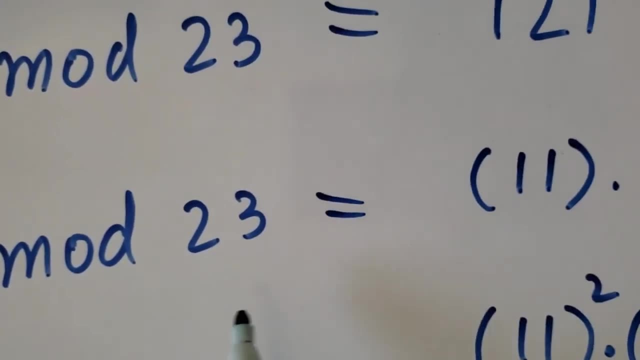 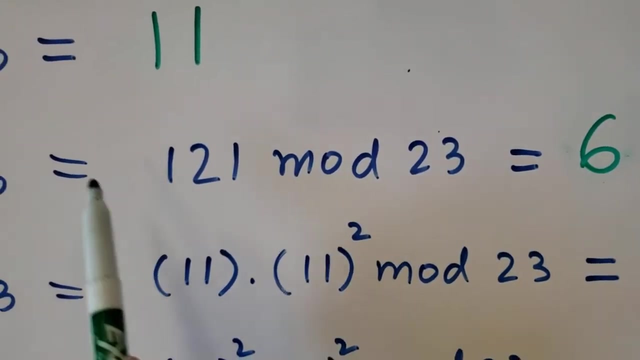 11 to the power 2 mod 23 is 121 mod 23, which is 6.. 11 cubed mod 23 is the combination of 11 times 11 squared mod 23.. We already calculated the value of 11 to the power 3 mod 23.. 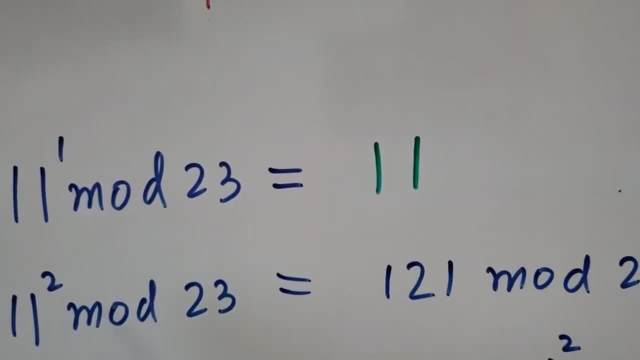 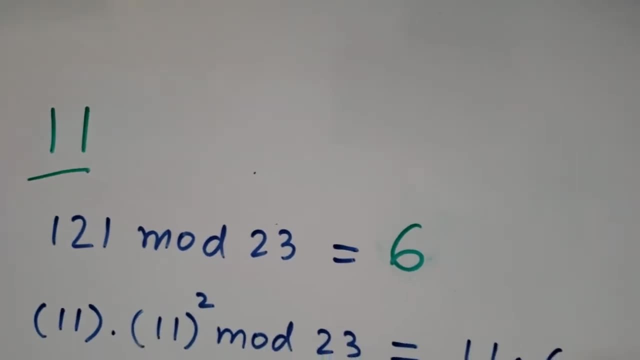 We will calculate the value of 11 to the power 2 mod 23, which is 11, and 11 squared mod 23, which is 6.. So we will take the value 11 from here and 6 from here. 11 times 6 is 66. 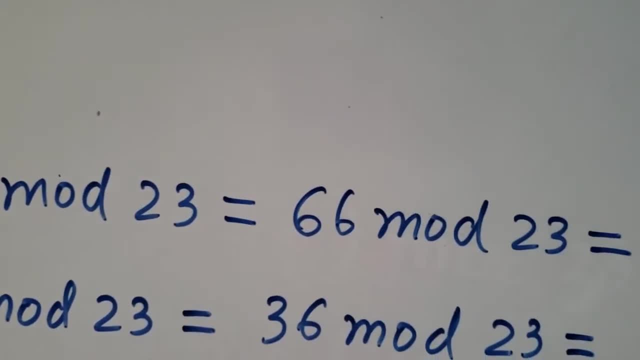 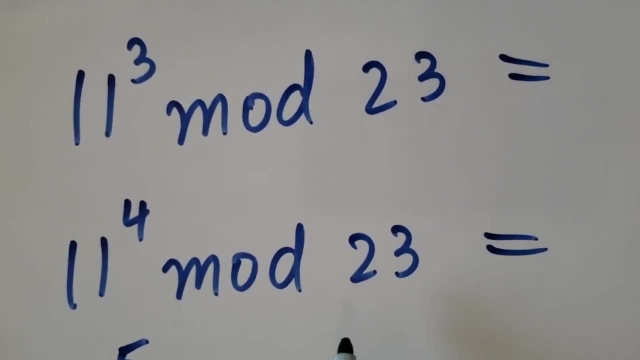 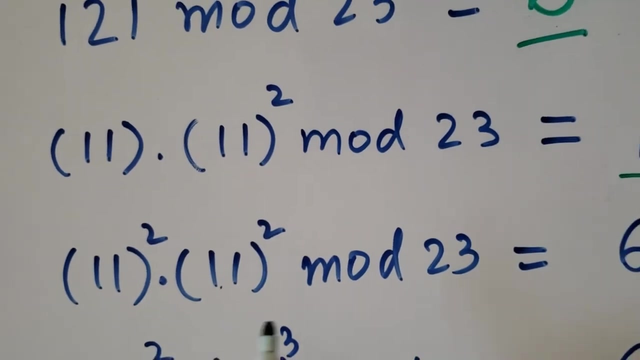 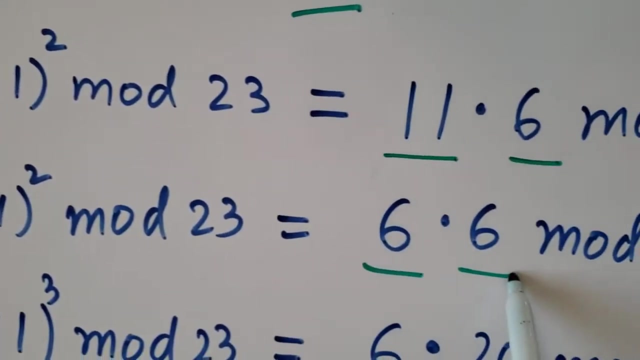 and we'll calculate 66 mod 23, which is 20.. All right, now we'll calculate 11 to the power 4 mod 23, which is again a combination of 11 squared times 11 squared mod 23.. square mod 23.. 11 square we already calculated as 6 here. So 6 times 6 mod 23 is 36 mod 23, which is: 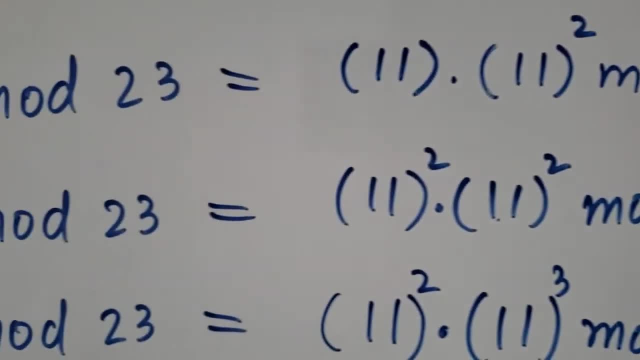 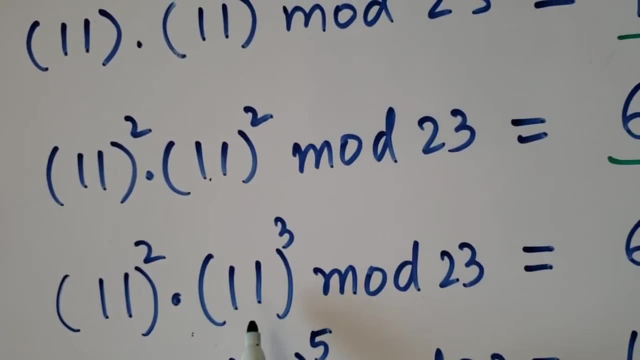 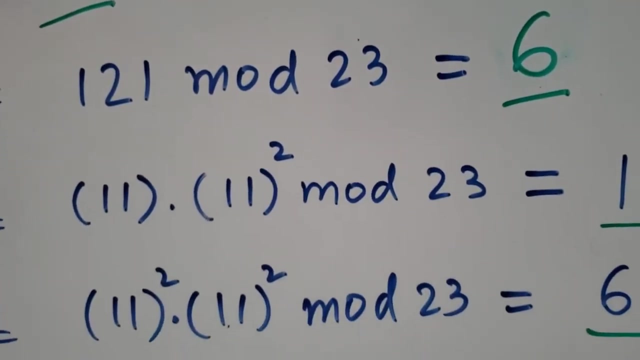 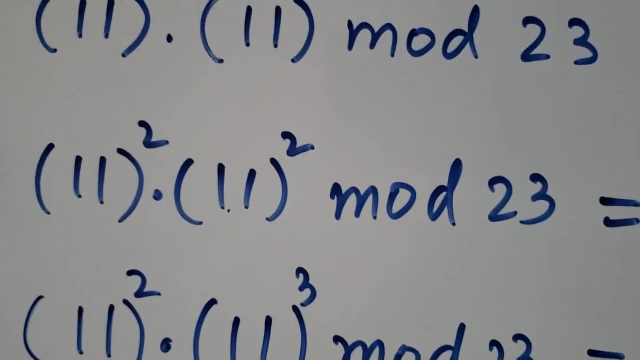 30.. Now 11 to the power 5 mod 23 is a combination of 11 square times 11 cube mod 23.. 11 square is 6, we already calculated here, and 11 cube, we calculated here here, 20.. So 11 square times 11. 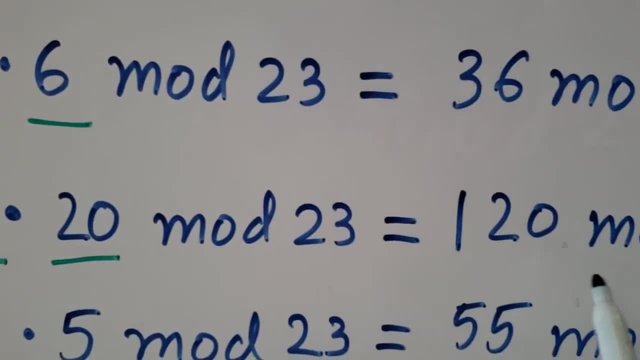 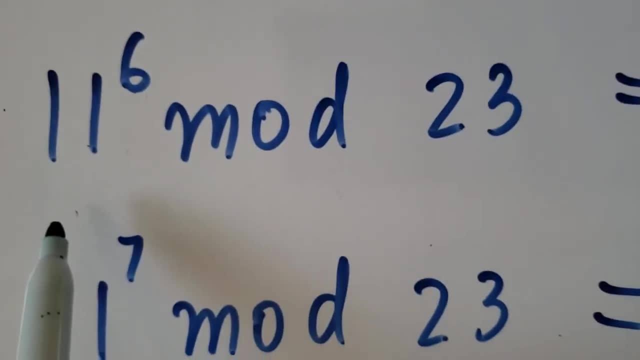 cube, mod 23, which is 120, mod 23, which is 5.. 11 to the power 6 mod 23 is a combination 11 times 11 to the power 6 mod 23.. So 11 to the power 6 mod 23 is a combination 11 times 11 to the power. 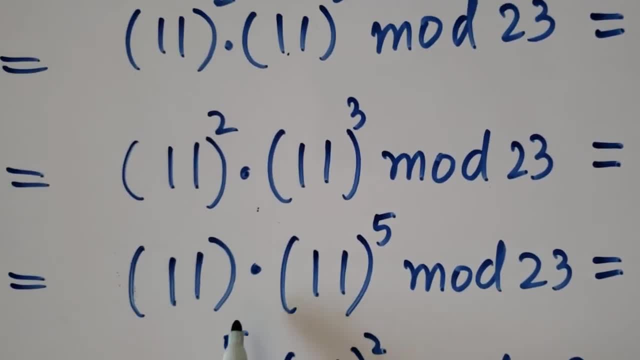 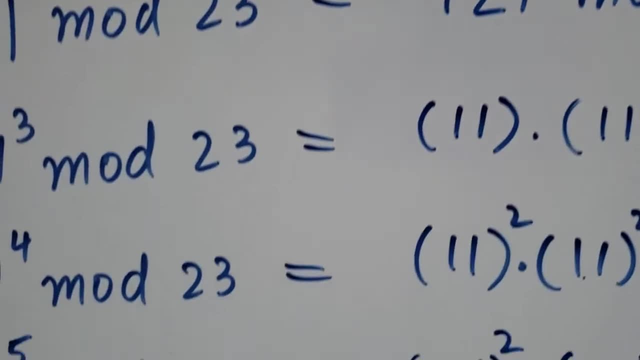 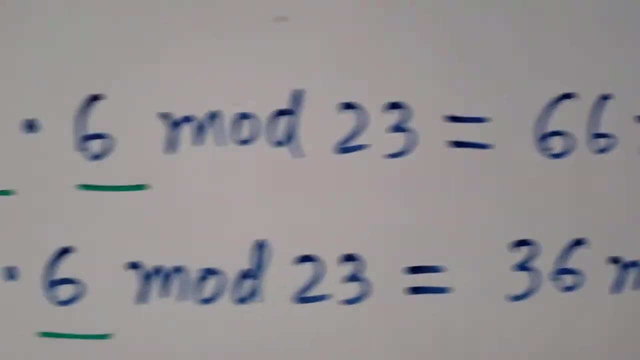 5. Why I am taking this combination. You can see 11 to the power 1, mod 23 is 11 and 11 to the power 5 is 5, which is a small number as compared to 13 and 20.. That is why I am taking the combination. 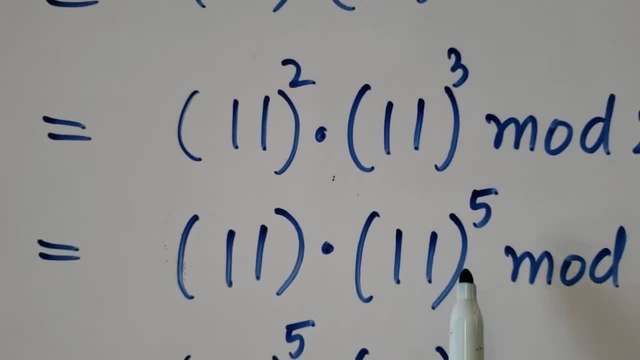 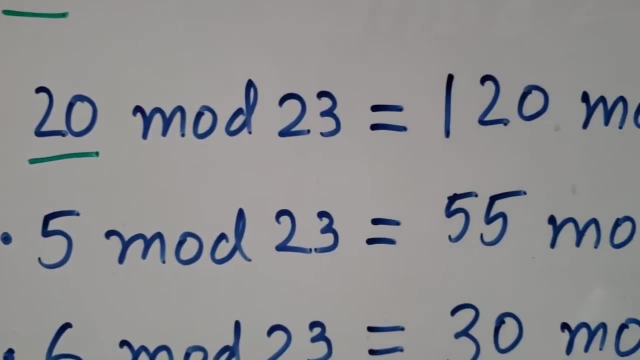 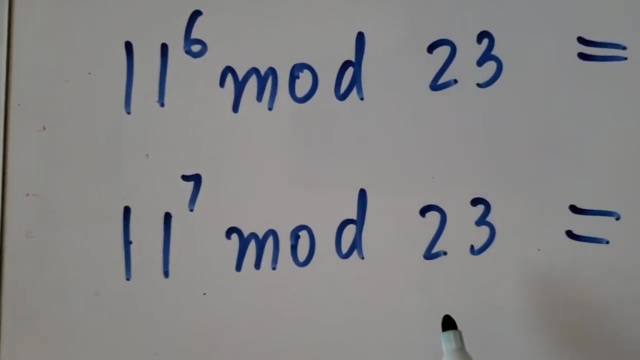 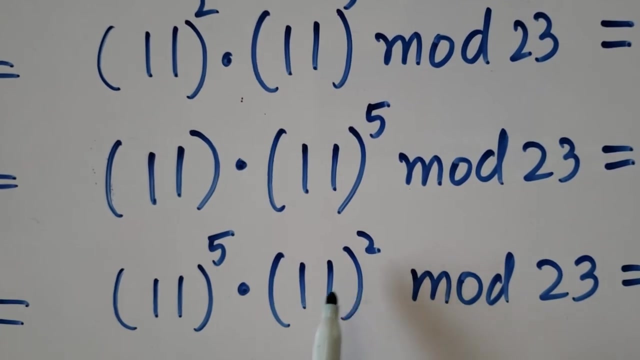 of 11 to the power 1 times 11 to the power 5 mod 23.. The multiplication of 11 times 5 is 55.. 55 mod 23 is 9.. Now, 11 to the power 7 mod 23 will take the combination of 11 to the power 5 times 11 to the power 2.. 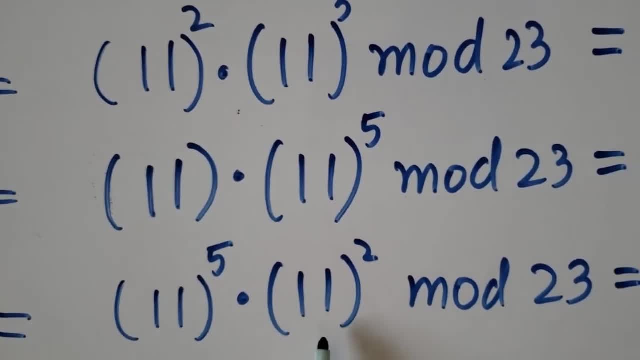 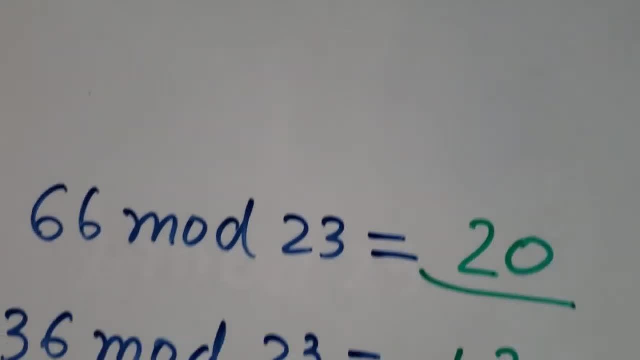 Because 11 to the power 5 is 5 and 11 to the power 2 is 6. both of these two numbers are smaller as compared to 20,, 13,, 9 and 7. So depressed on the other side and esteemed to know the further questions Here are. the third number is 16.. This number has multiple numbers, which gives each of those two 25 plus 7.. Both of these numbers are equal in size. If you forget to mention them, then you have to skip till 1 to метre, or 1 to the power, 12.. So now E's given. here we have 25 plus 25 is 17, which is 9.. But in the end you have 50 plus 11 plus и 11 to the power 7. mod 23 is 9 and 11 to the power 5 and 11 to the power 2 is 6.. 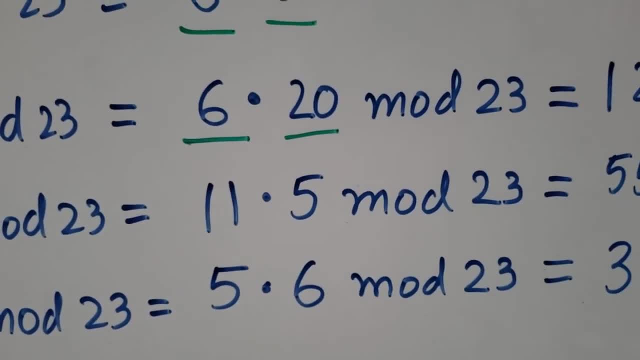 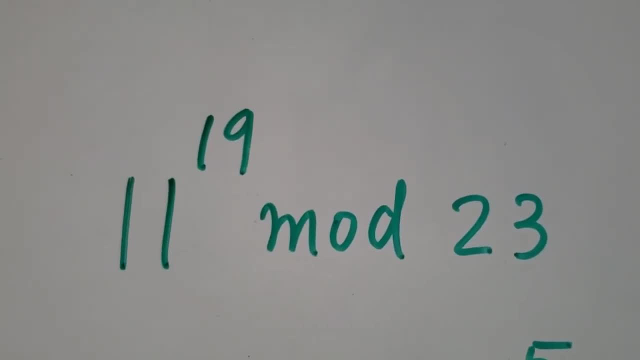 of 5 and 6 is 30. 30 mod 23 is 7. let's look at the problem. 11 to the power 19. that can be written as 11 to the power 7, square times 11 to the power 5, mod 23. we. 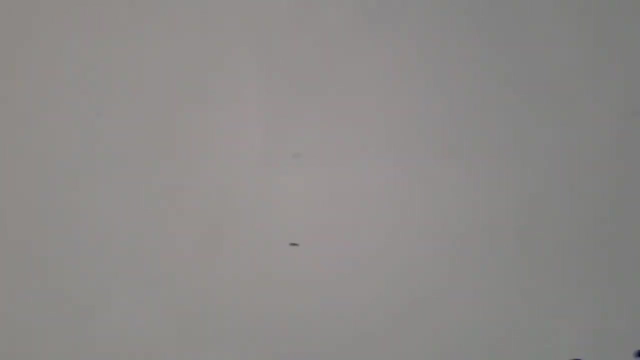 can also use other combination like 11 to the power 8, square times 11 to the power 3, mod 23, but for this you have to calculate 11 to the power 8 and you have to calculate one more step. so that's why I'm not going to use this combination. 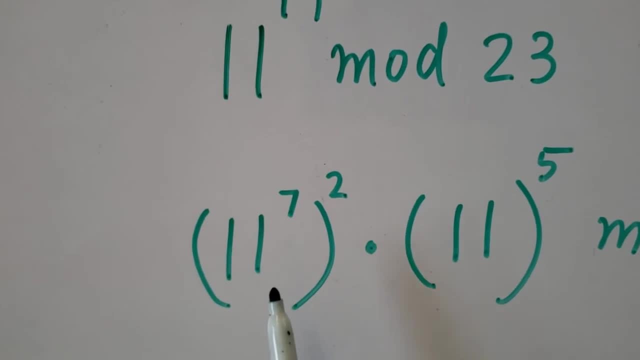 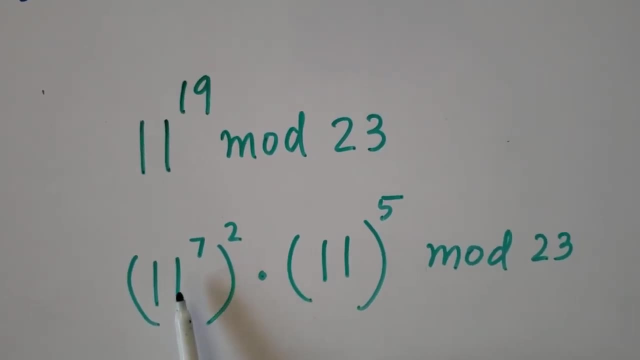 I'm going to use the combination: 11 to the power 7, square times 11 to the power 5. why I'm using this combination? as you can calculate here: 11 to the power 7, 7 times 2 is 14, 14 plus 5.